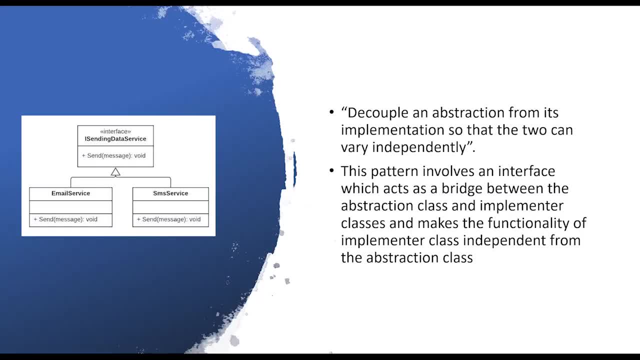 email, sending SMS, for which we can write their own implementations. Now suppose that there's a requirement of orthogonal class where we need to send data using a separate service. Up till now, suppose, say, we were using one service, say web service, But now a third. 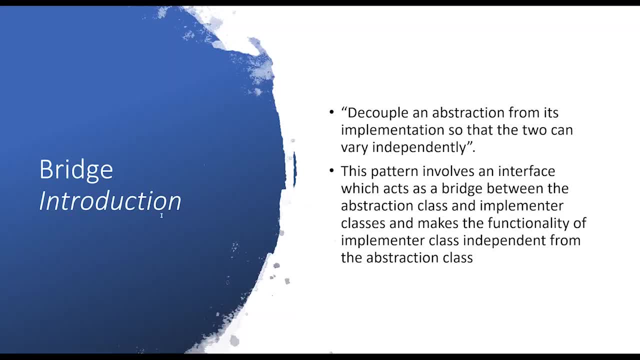 party library orthogonal class, which I said. that is means you can say a different dimension, which is a dimension not relevant to ours, Like, suppose, sending data, that is one dimension we can see, but the service which we are using to send the data, that may be a different dimension. 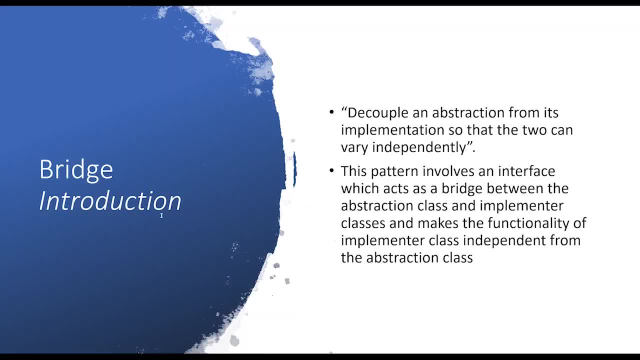 that means a separate concerns analogous to real life definition. You can say that TV and remote. TV is Wan implementation and remote is a separate kind of thing. Ah, similarly we can have switch and it's the electronic equipments Did. these are two orthogonal dimension. 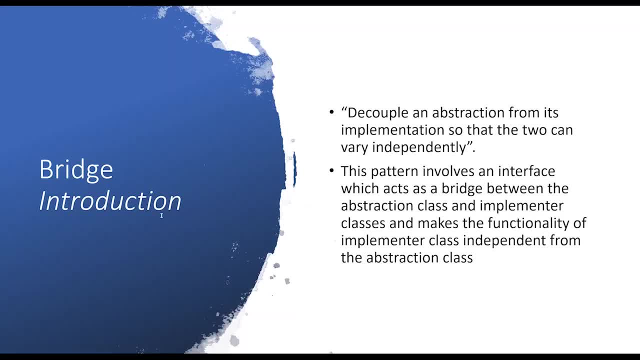 of things, keeping the congruence right. Yeah, Kind of You will say that. So so up till now, suppose we- yeah, we- are sending the data using web service. Now suppose we are just a second. Now suppose we, in our application we have integrated with a third party library and 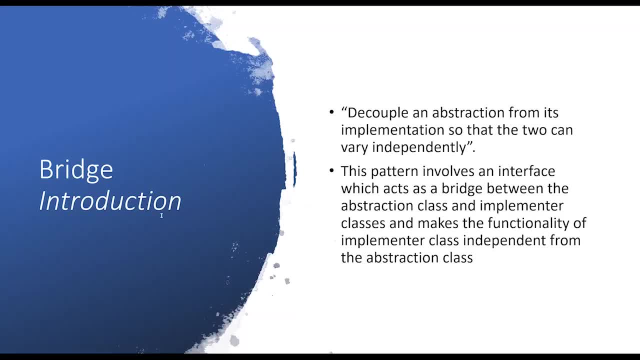 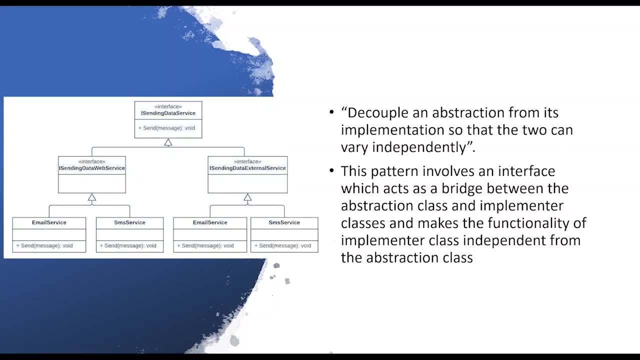 we want to send the email and SMS, all those, whatever the mode we had. we want to send those data with the same mode but using a different library. This means that we will have to double our implementation, which should be send email using a third party library and similarly send SMS service using a third party library. 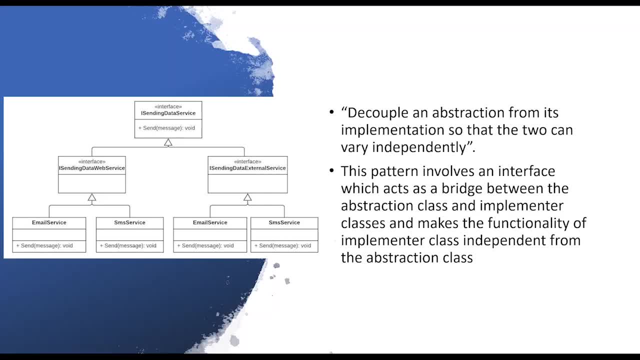 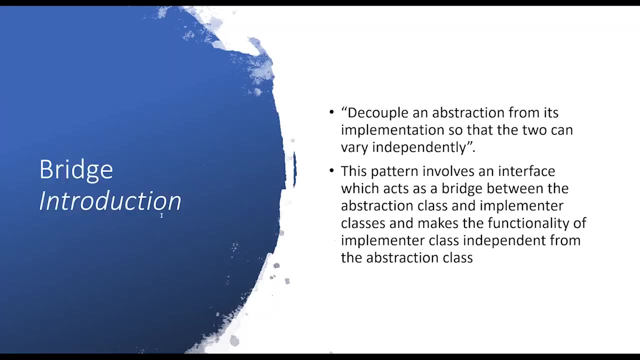 This is the problem. which rich pattern will come in picture to solve. this means what was the problem? again, the problem was like: with each addition of the dimension, we will have to, exponentially, we will have to add classes. we will have to continuously extend classes using the inheritance, in the inheritance way. 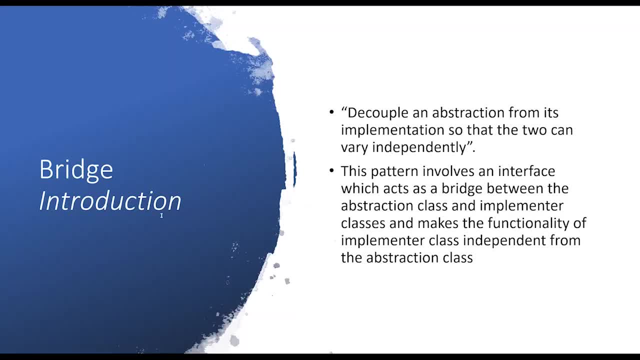 Like, suppose now a separate mode of sending data arises, like, say, earlier we were having email and SMS. now suppose, just suppose, say, postal service, Something out of that, not saying that or call. yeah, so exponentially we will have to implement it both for the web service and the third party library. we will go after that. 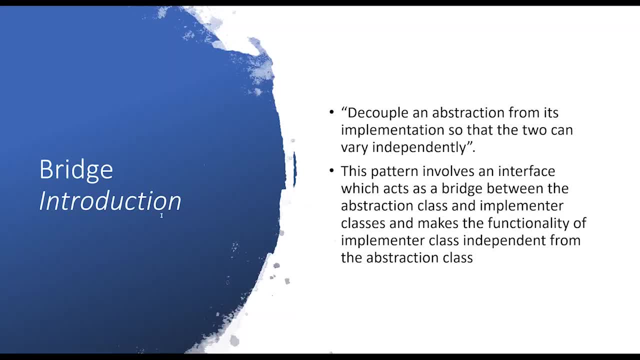 So this is the problem which arises in the inheritance, that for every dimension we will have to extend it. actually, the problem here is, like the compile time binding of the base class, which is the sending data, which is with their actual implementation. first of all, let's reiterate: 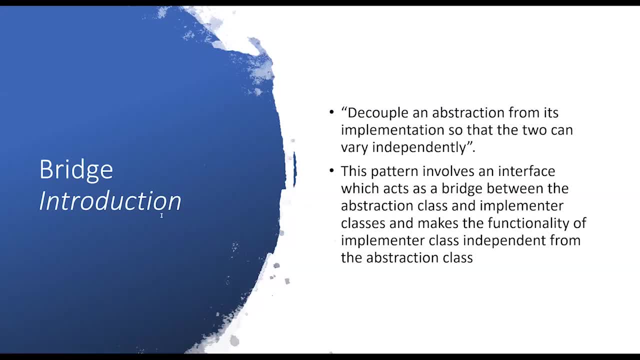 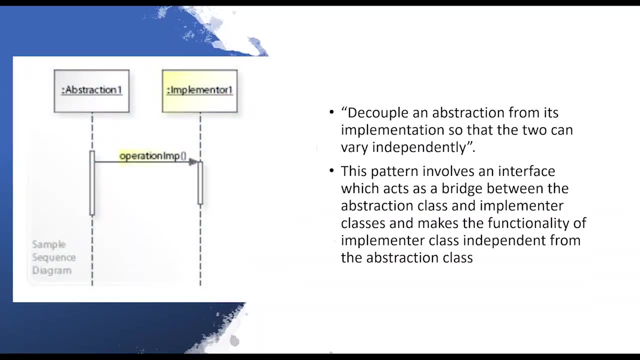 What is the standard definition given by the Ganga force? here they are saying: decouple an abstraction from its implementation so that the two can vary independently. And so what they're trying to do is separate the abstraction in the implementation part in their own hierarchy. in simple terms, instead of following usual inheritance we will create. 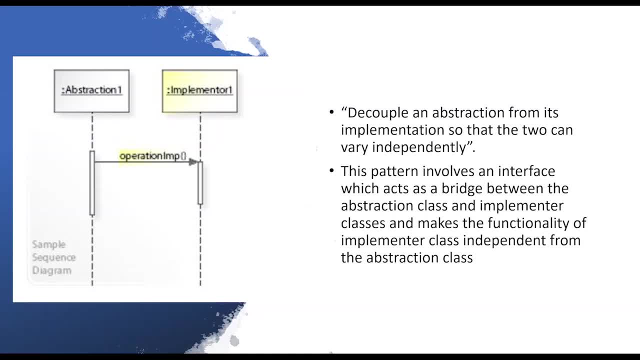 a separate class of abstraction and separate for inheritance, which will have their own implementations, again in terms of previous example of mode of sending data using different service. the bridge design pattern proposes refactoring this exponentially explosive inheritance hierarchy into two orthogonal hierarchies. separate out the two hierarchies: one for service. 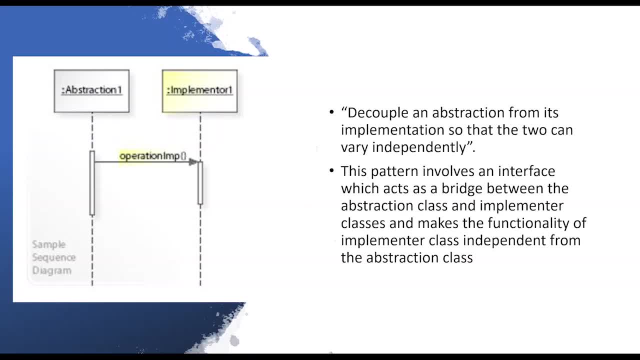 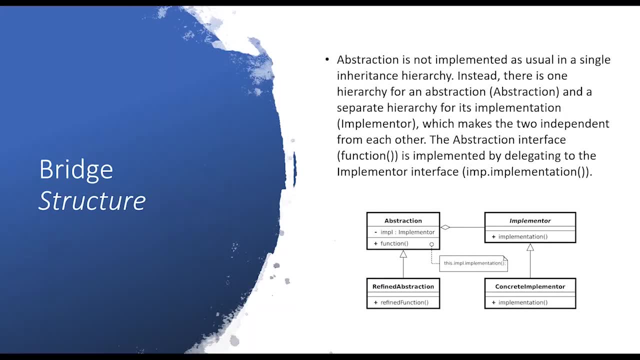 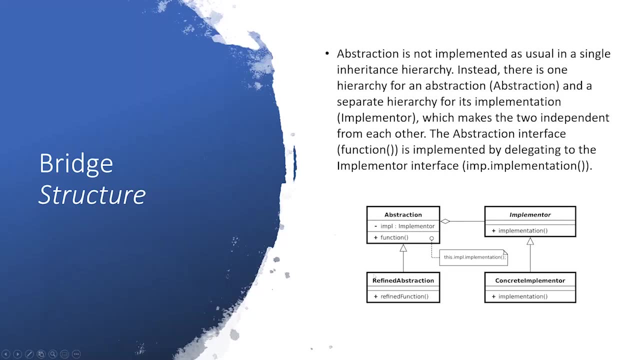 independent abstraction and other for service dependent implementations. so what we are trying to do here, Like We will create, as shown here in the class diagram. here what we will do, we will create a hierarchy, inheritance hierarchy for abstraction itself and a separate hierarchy where the actual implementation is happening. they will have their own hierarchy. so at the run time, 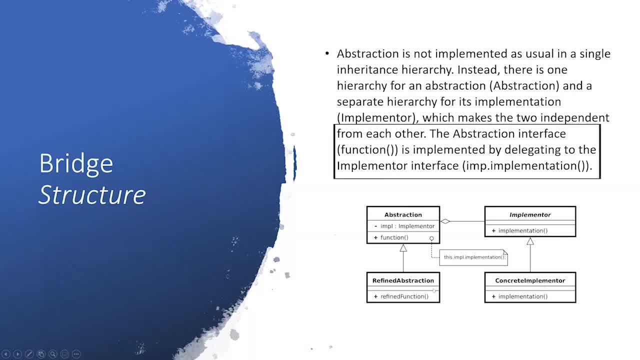 what we can do. we can run time. we can bind which abstraction will be working with which implementation way. so means at run time we can decide: send SMS. we want to send SMS using web service or third party API. we are dynamically binding our implementer to abstraction here. 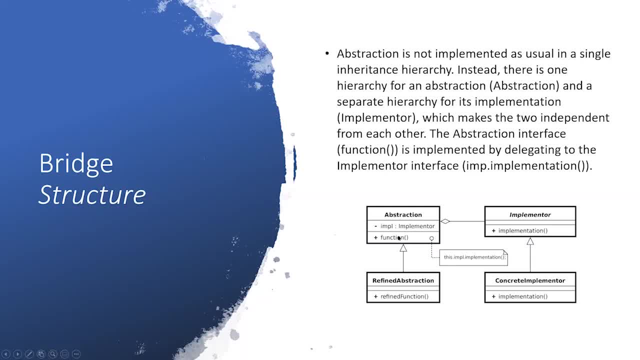 and finally, from the function. what will the function do? function will do nothing, but it will be calling the implementation property, implementation method of the IMPL which it is composed of. so what we have done here, we have separated out one dimension, separated out the other dimension. 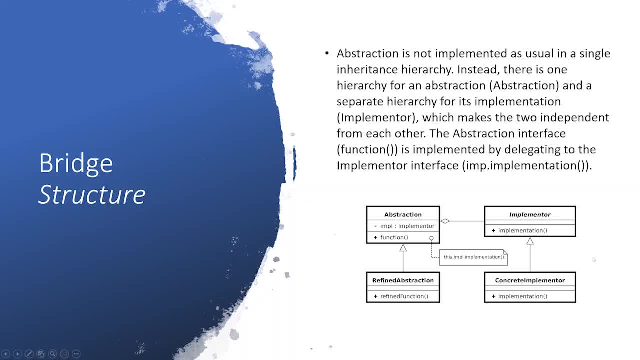 Separated out: this dimension, we will deal with sending data, and this dimension we will do. we will deal with which web service we want to use. so at run time we can define: send SMS using web service, send SMS using, say, third party library. okay, so what is the solution? 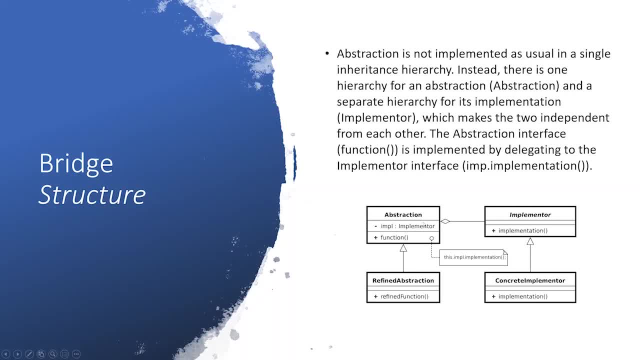 here is. we will separate out. we will create a bridge here, So We will. This is the bridge which, from which the name comes, abstraction, abstraction or implementation. abstraction inside will compose of the IMPL property, which is the implementer interface object. yeah, and this is so at runtime we can define which implementer it wants to use. let's. 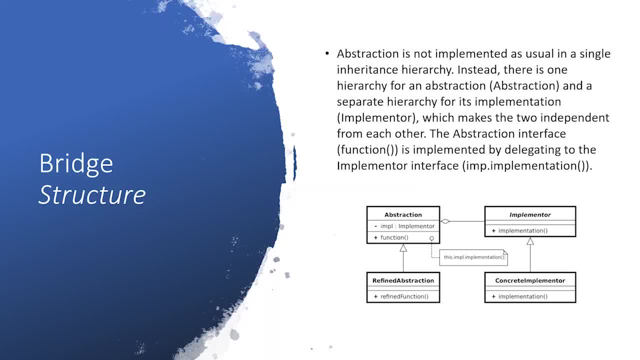 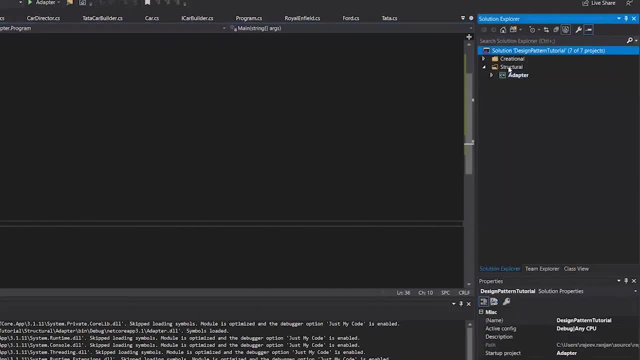 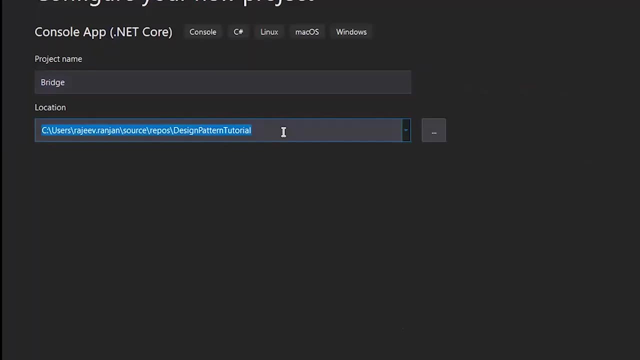 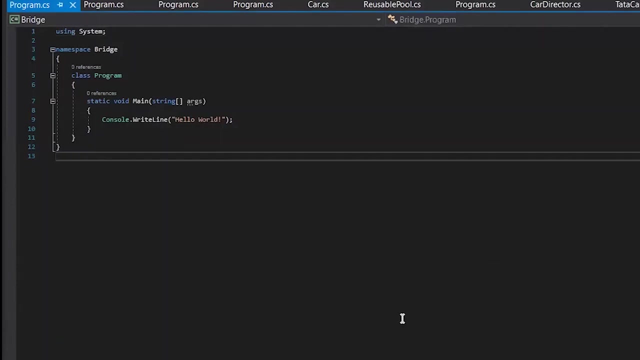 try to go into the code to see how it is working means. I think that would be much more beneficial for you to understand. Let me add a project here. Okay, so I'll be creating a structural bridge Create. So this is our another console application. you can see so in this console application. 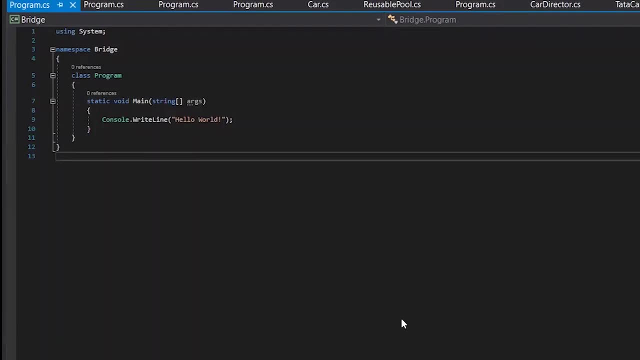 let me try to implement what is happening here. First of all, let's try to understand what is happening here, So in this console application. let me try to implement what is happening here. So let's try to understand what was the problem. okay, in fact, that would be much more beneficial. 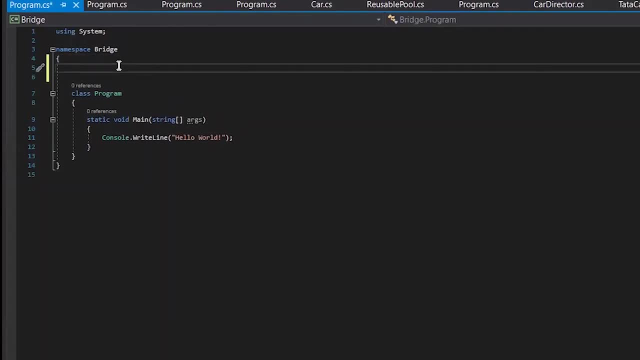 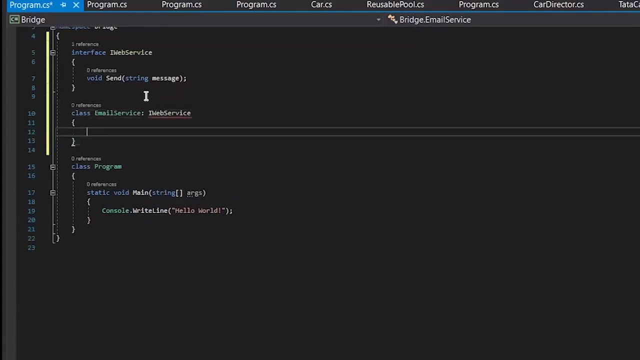 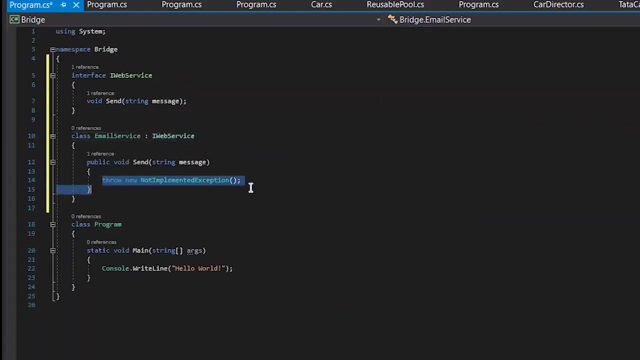 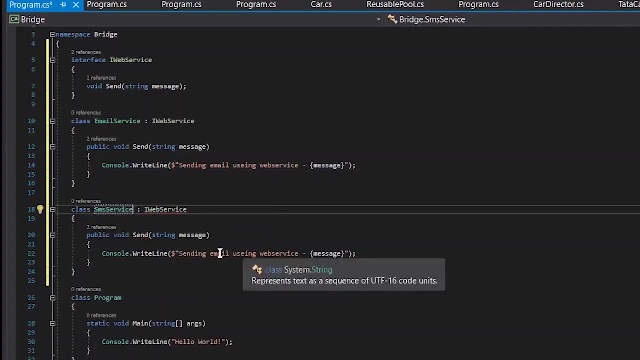 let me for create interface I web service. so this is our interface and I will implement class email. I'll implement the interface. I'll just write, I'll just print out a line: consoleWriteLine. This will be our implementation of the email service. uh, SMS service: sending SMS. okay. 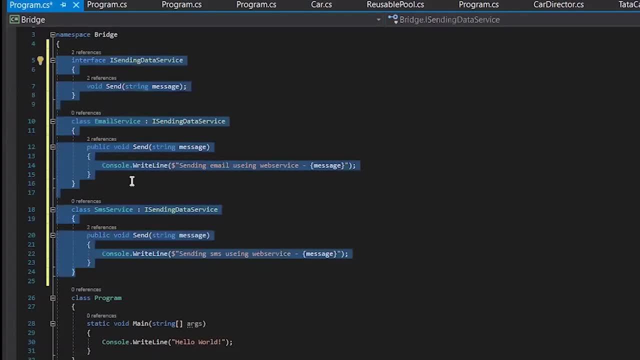 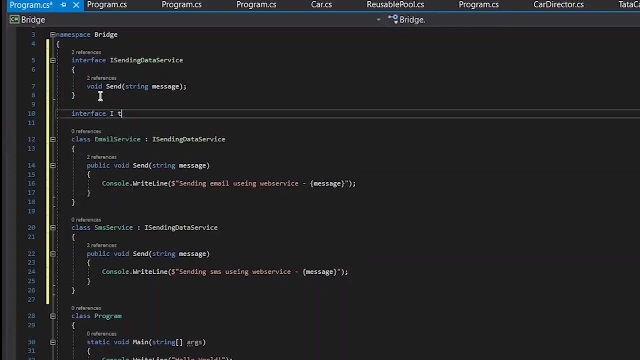 So what is the? this is a simple inheritance scenario where we are doing this. Now suppose another third party asset, a third party library, comes, then we will have to create a separate interface- uh, I interface, uh, I third party library- which will have 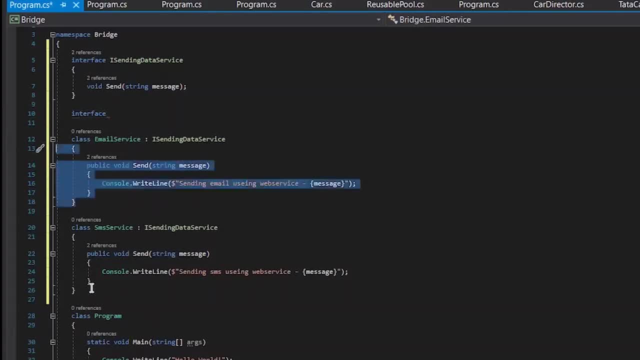 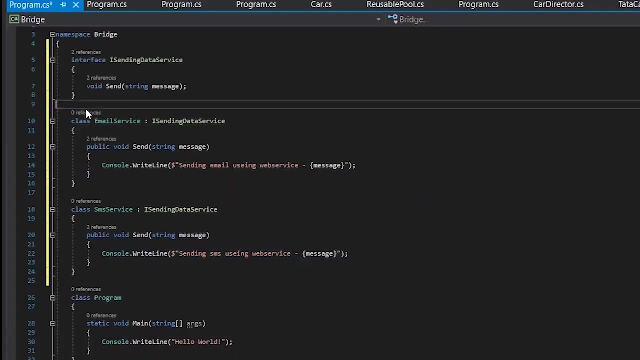 its own white send and duplicating this class with the justice. uh, the implementation strategy will change. Right there, We will write: sending SMS using a third party, sending email using third party. So you see, uh, We are binding the compile time. 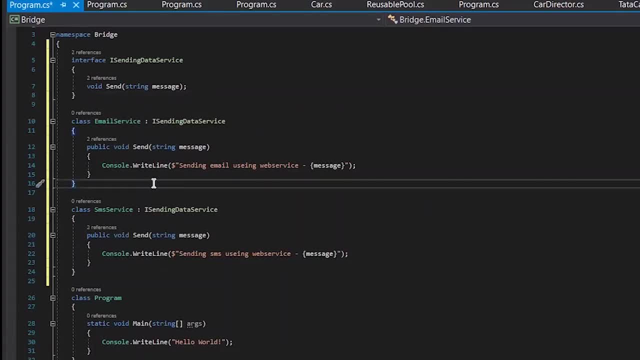 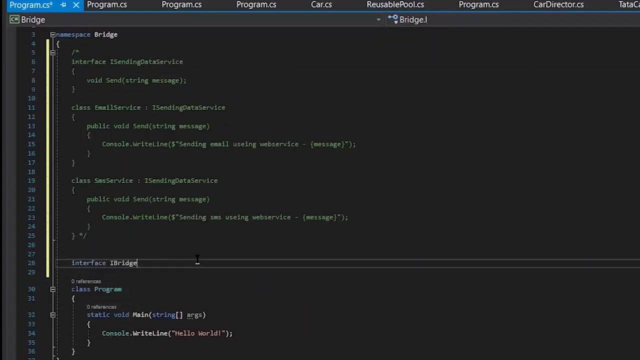 Uh, we are binding our abstraction with the compile time. Uh, let's try to understand how. how the? uh, let's try to refactor it according to the bridge design pattern. Okay, According to this pattern, we need to base classes or interface, which will be our pillars. 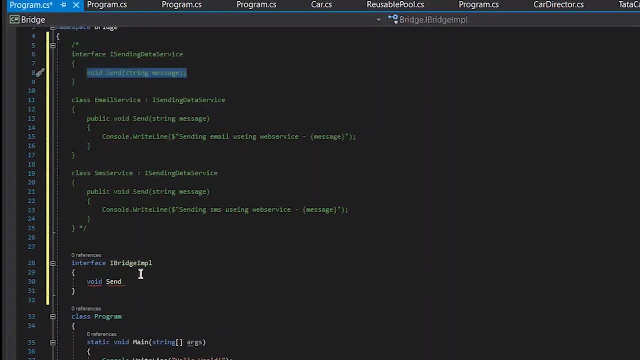 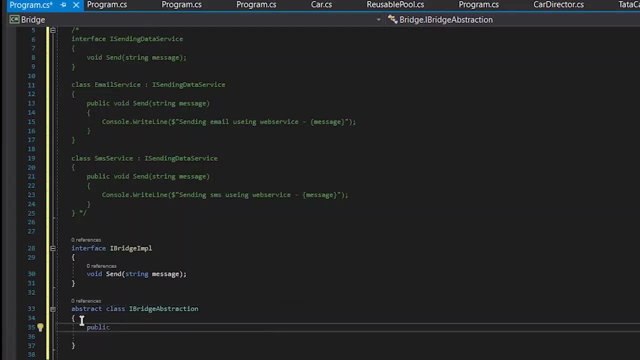 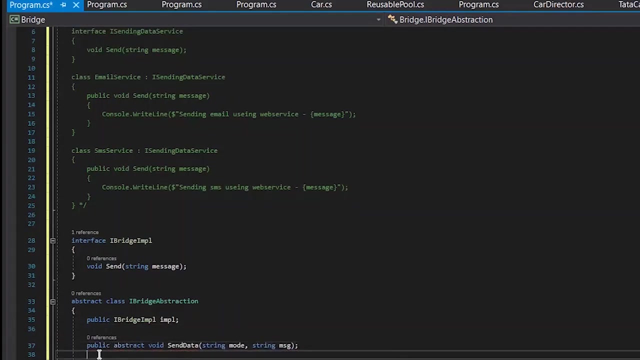 of the bridge, One for abstraction and the other for implementation. This is what I'm creating here. Okay, So we have created the two separate base classes, which are one. our abstraction will be, uh, extending this. our implementation will be extending these. 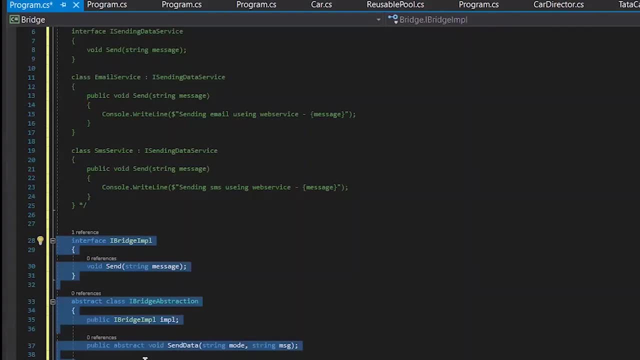 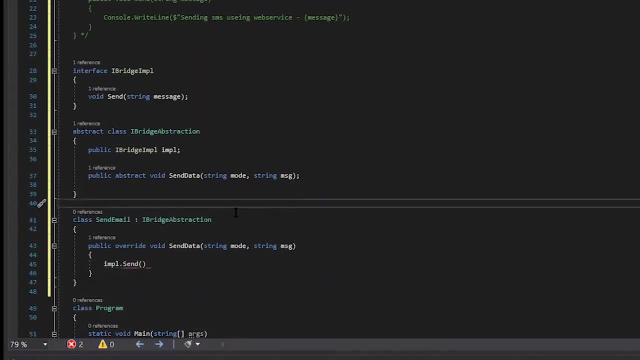 let's state our concrete abstractions, which will be send email and send SMS, which are dealing with the modes by which released And data internally. they will be calling the actual implementation, which is I, MPL 돔send, with the mode as a parameter. 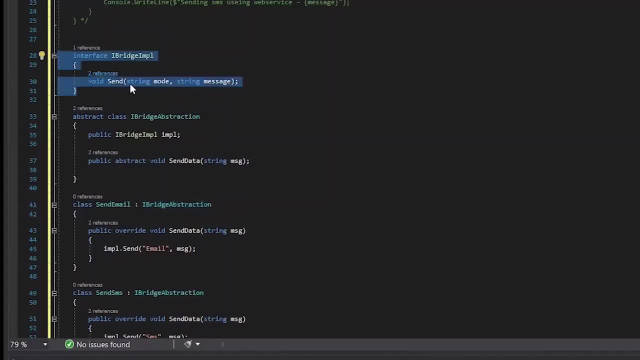 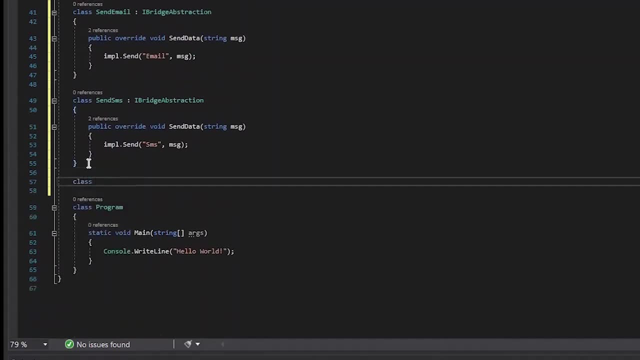 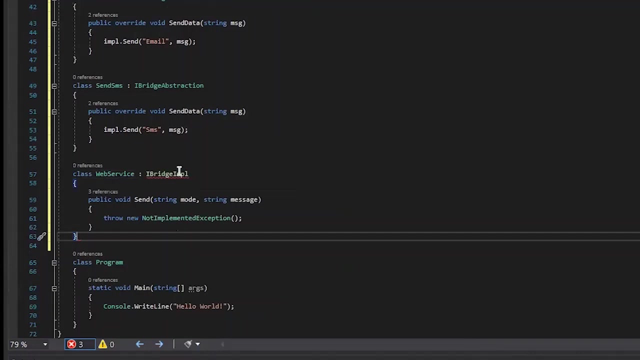 And our implementation will be actually implementing this eyebrows IMPL. So let's Do the actual implementation of this. I'veeso MPM Plus. uh, uh, uh, uh, a web service. I bridge, I MPL, and inside this I will be writing console dot write. 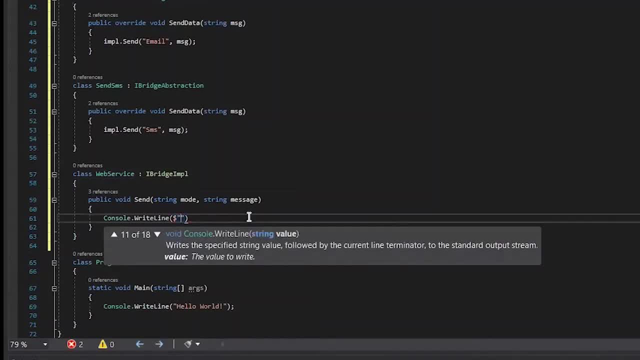 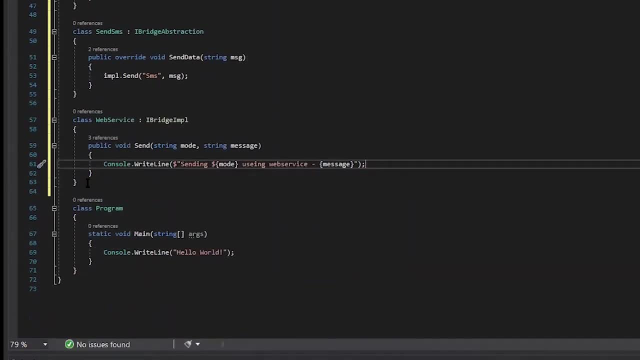 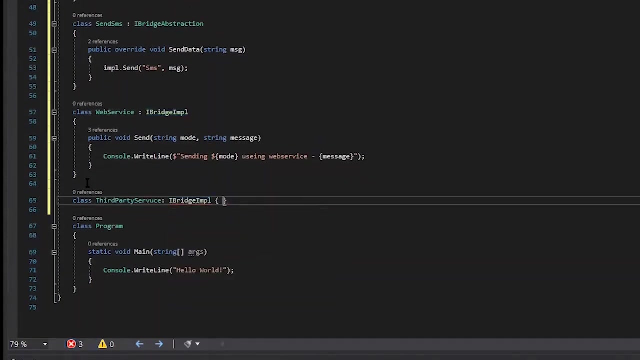 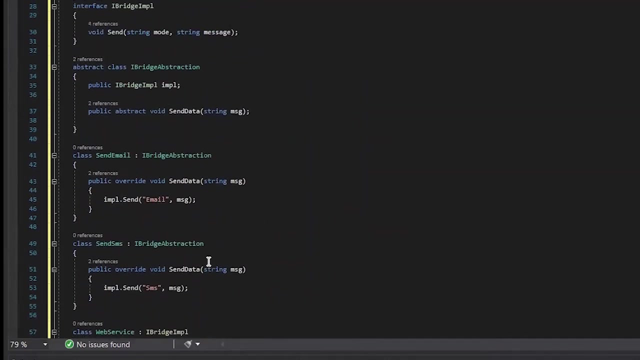 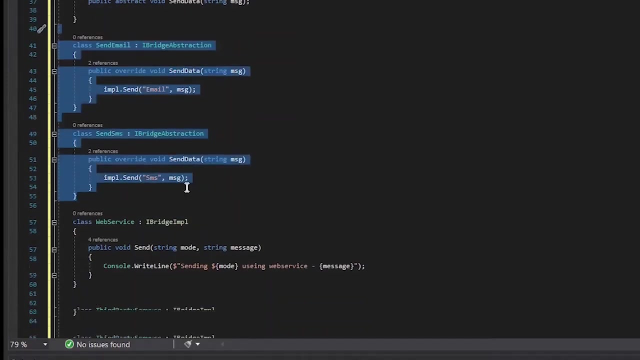 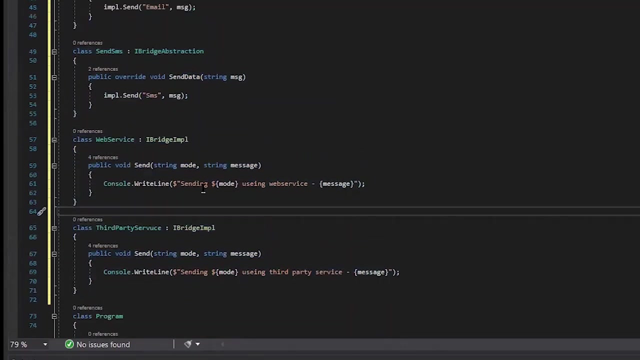 line class art party, this service. I am pure IMPL and similarly it will be sending mode using service. so you see, we have separated out the concerns here. we have separated our one concern for email in a separate classes and our concern for with service to use in the separate classes. so suppose any 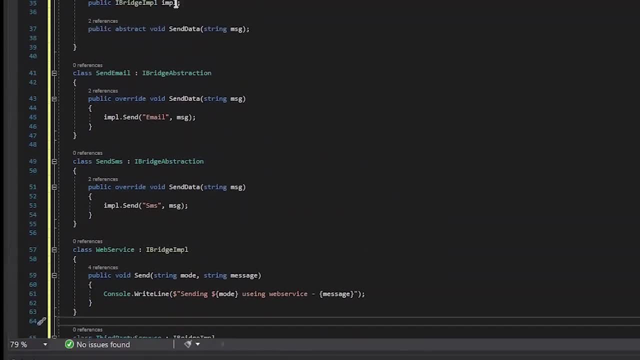 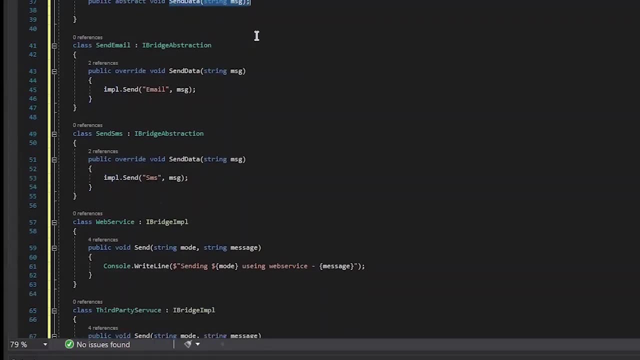 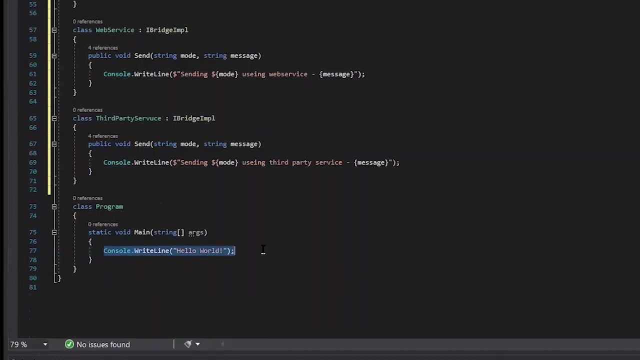 future implementation may come. suppose a future deployment implementation come, we just need to bind this IMPL separately and we just, similarly it will follow the same protocol. just try it out in our client library to have it to see what is actually how it is behaving properly. which abstraction service. so at runtime I'm deciding which email I want to send. I can. 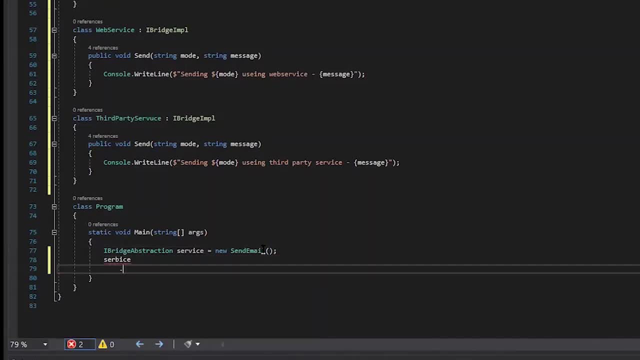 decide and at runtime I can decide service, service dot. at runtime I can decide which service I want to use. I can use third party service or I can use web service. and finally, to actually send the data, I will use service dot: send data. hello world. let's just try to run this application to see if 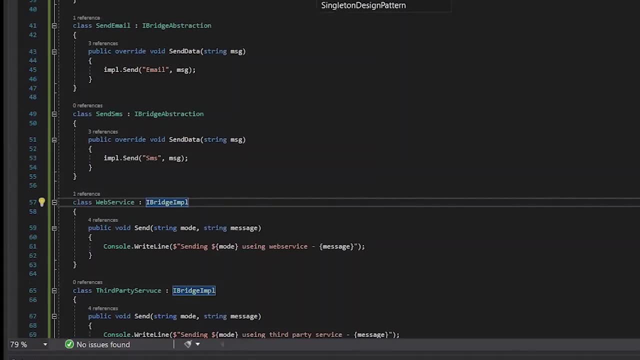 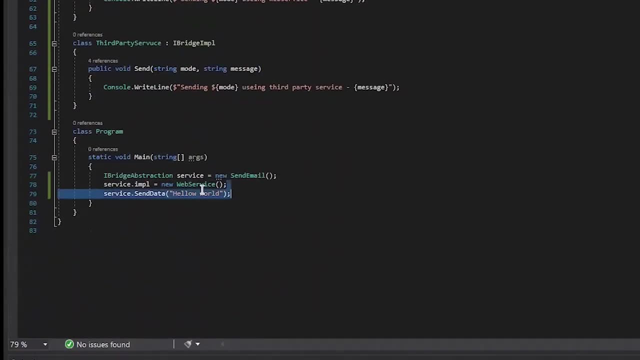 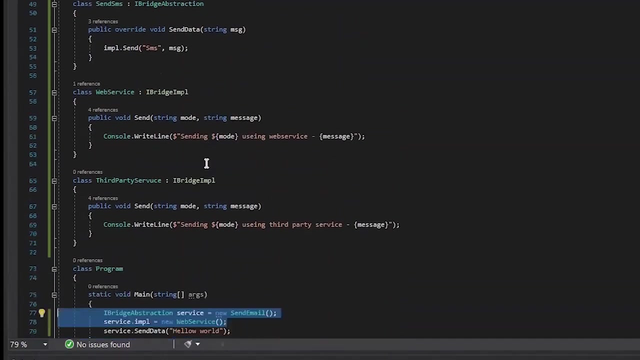 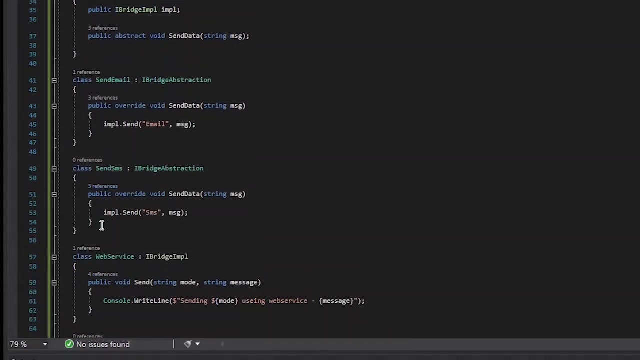 any issues there. with or not, you can see the same output. we are sending email using web service, hello world. and this all we can decide at the runtime which we want to use, without any consideration for the previous separate dimension, or we can add our own service here. we can add our own separate service here, or we can separate. we can create our own different.